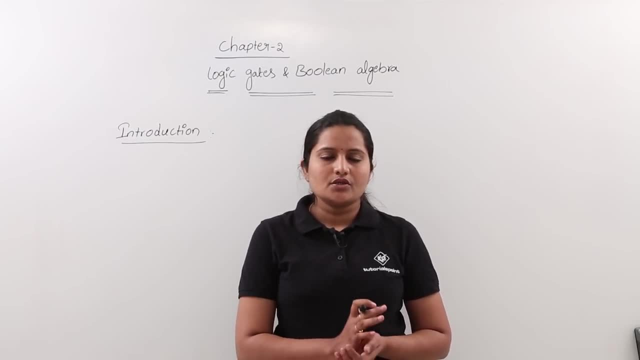 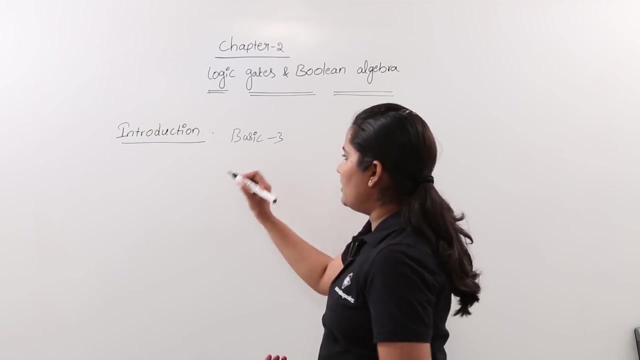 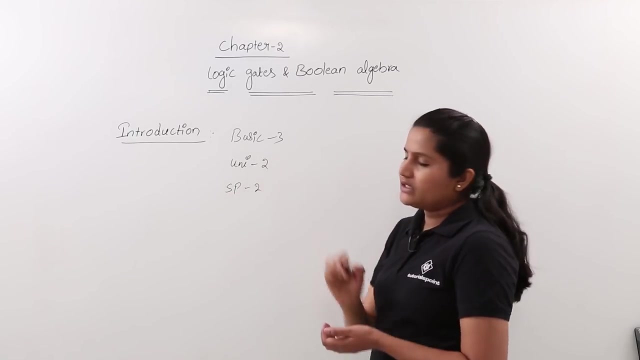 functions and used to provide single output. So here we are having three basic logic gates and two universal gates and two other special gates. So here we are having three basic gates and two universal gates, So, and two special gates. So these three basic gates are: 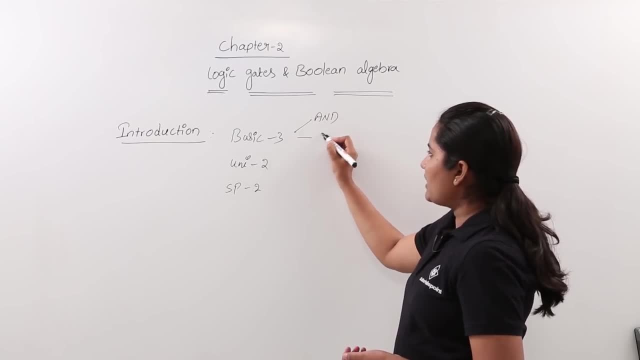 AND gate. next R gate and NOT gate. So these three are the basic gates And here two universal gates are NAND gate and NOR gate. NAND gate and NOR gate are called as universal gates Why? Because by using this NAND and NOR, we can implement all other gates That 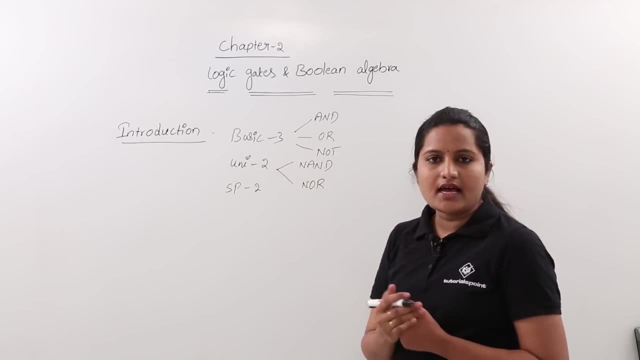 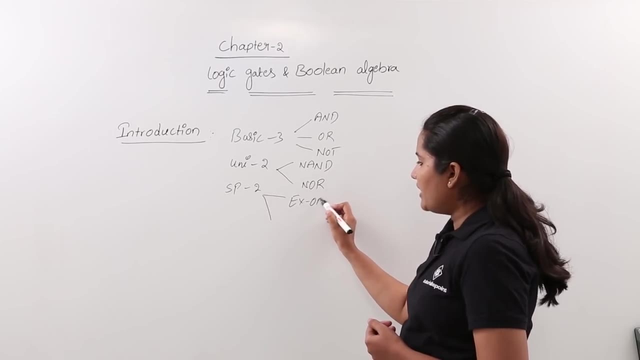 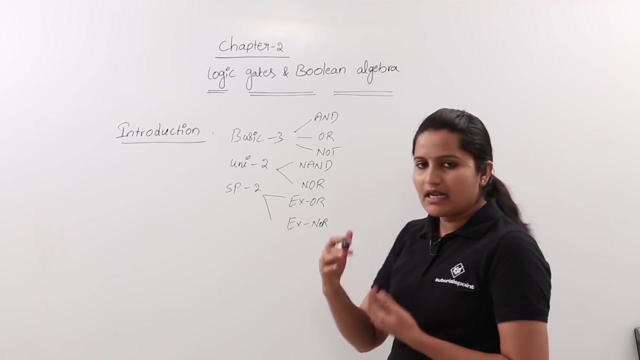 is why we are calling this NAND and NOR gates as universal gates, And you are having other two gates as XOR gate and XOR gate. So these are the universal gates. So these are the universal gates, XNOR gate. So these two are some special gates. We already discussed in last unit some 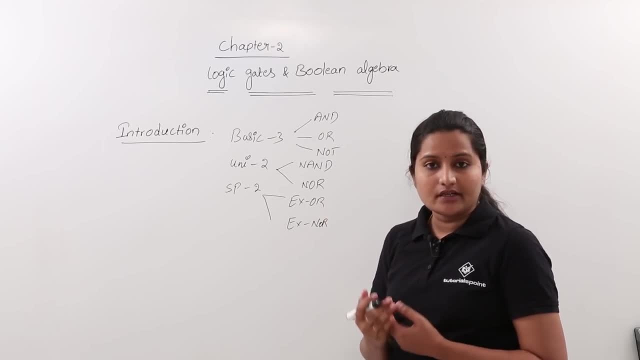 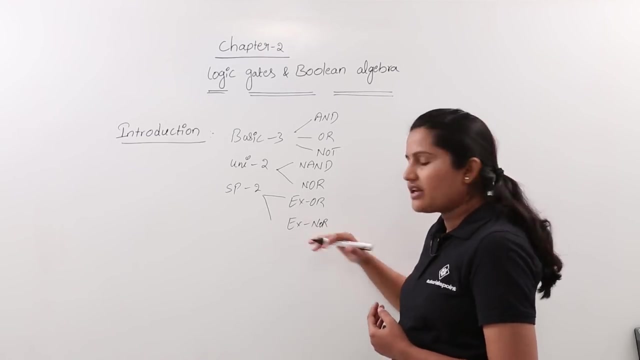 little bit about XOR gate. that is, this is a odd one detector. Whenever you are giving odd number of ones, it is going to provide high output or one as output At the same time. so here you can see XNOR gate. this is even one detector If you give one XNOR. 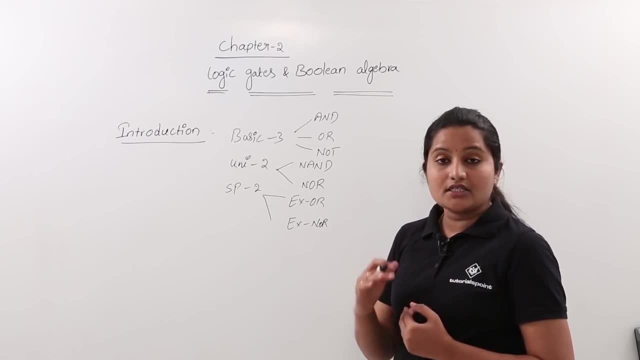 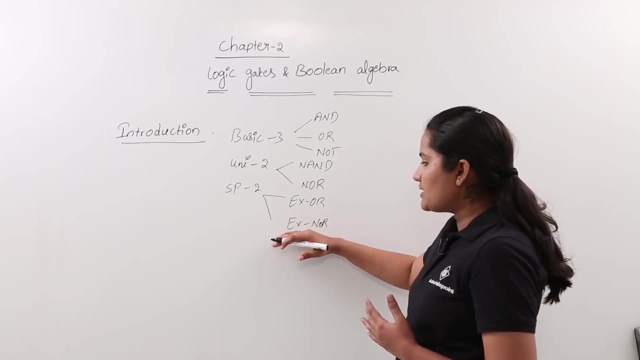 gate, this is even one detector. If you give one XNOR gate, this is even one detector, Even number of ones for XNOR gate, it is going to provide one there, It is going to provide one at output. We can say this is somewhat complement gate for XOR. So see here. So totally we are. 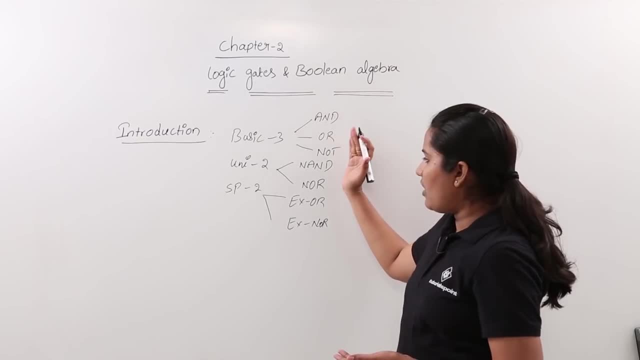 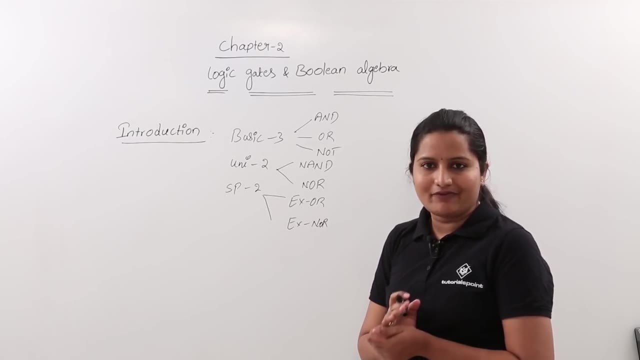 having seven gates AND OR NOT: NAND, NOR, XOR and XNOR. Now we will see the functionality of each and every gate here. Here, if you see this XNOR gate, you can see that XNOR gate is. 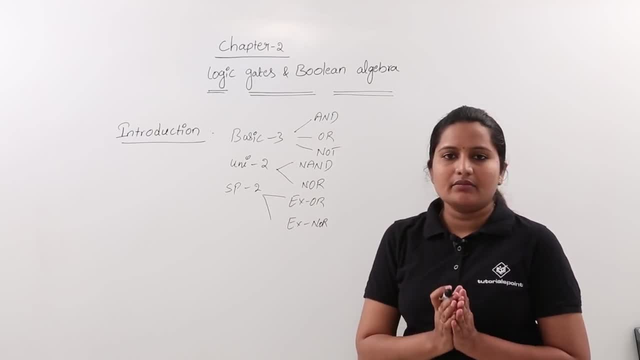 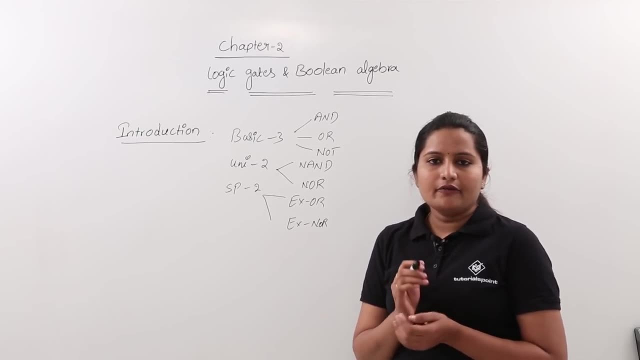 going to provide one XNOR gate. If you are having NAND gate means NAND is nothing but multiplication functionality. You just treat like multiplication functionality. For example, if you are having two input NAND gate, you may have N input NAND gate. but for example: 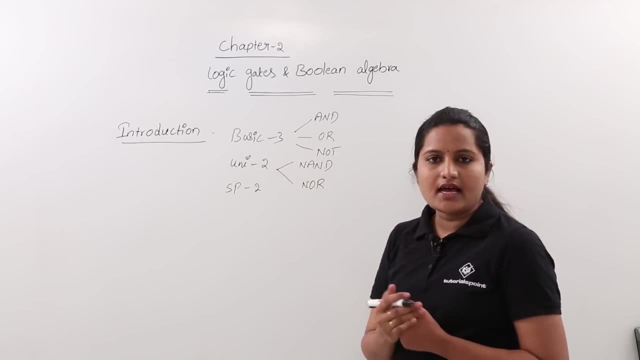 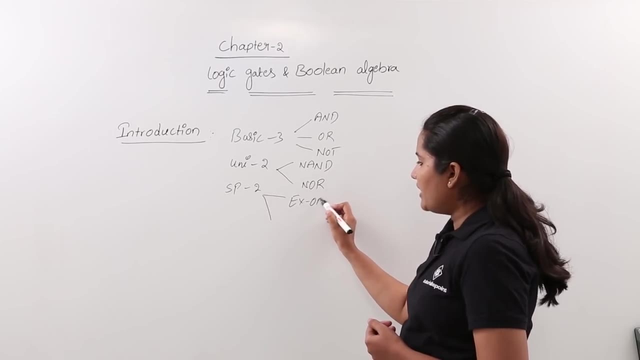 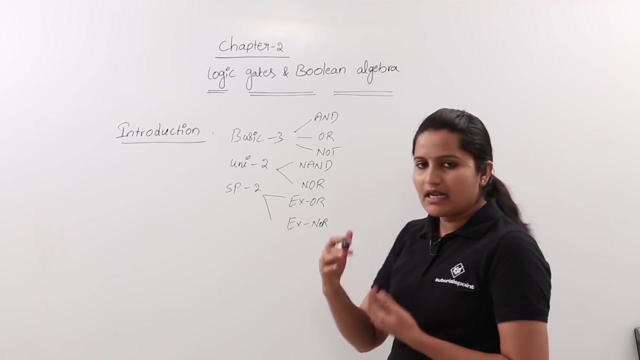 is why we are calling this NAND and NOR gates as universal gates, And you are having other two gates as XOR gate and XOR gate. So these are the universal gates. So these are the universal gates, XNOR gate. So these two are some special gates. We already discussed in last unit some 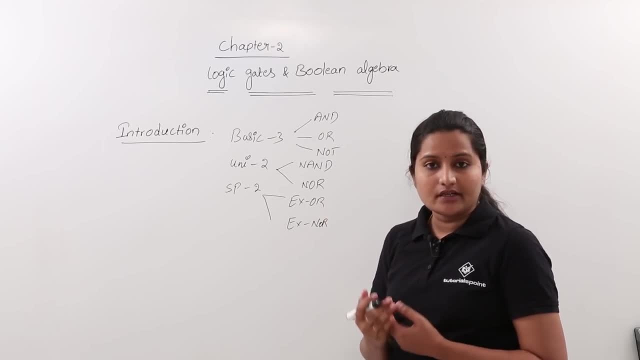 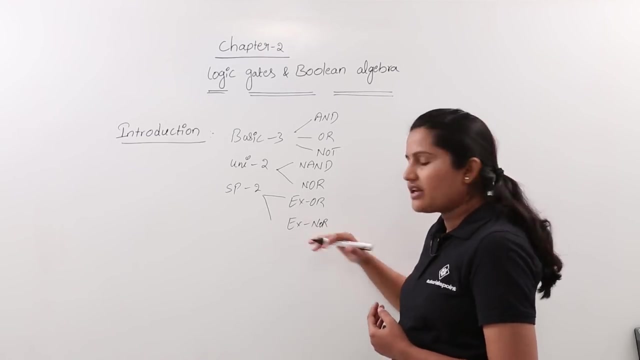 little bit about XOR gate. that is, this is a odd one detector. Whenever you are giving odd number of ones, it is going to provide high output or one as output At the same time. so here you can see XNOR gate. this is even one detector If you give one XNOR. 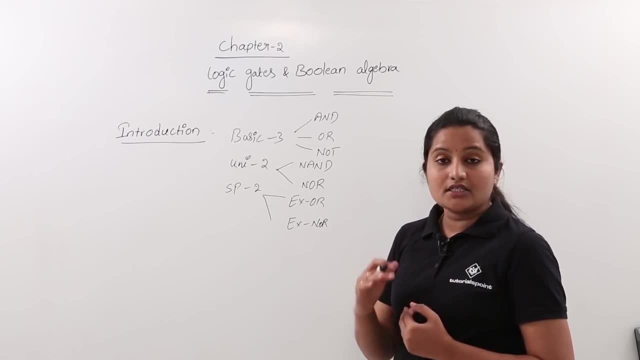 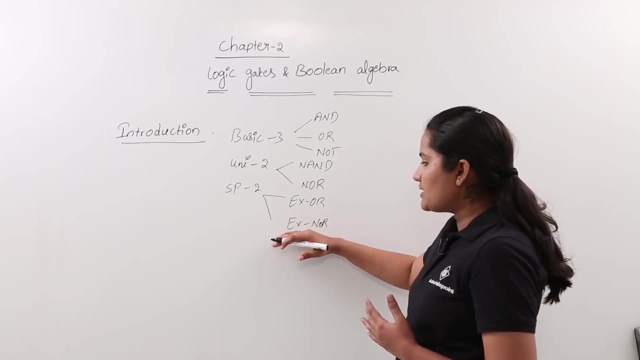 gate, this is even one detector. If you give one XNOR gate, this is even one detector, Even number of ones for XNOR gate, it is going to provide one there, It is going to provide one at output. We can say this is somewhat complement gate for XOR. So see here. So totally we are. 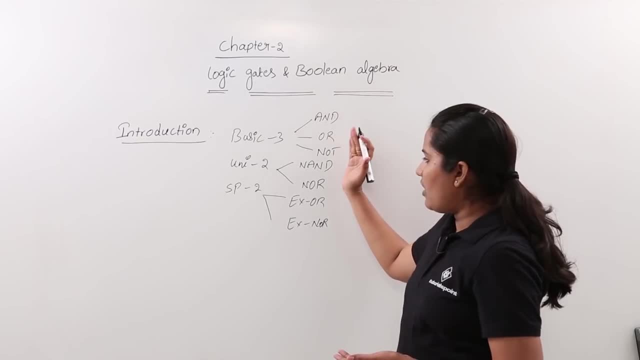 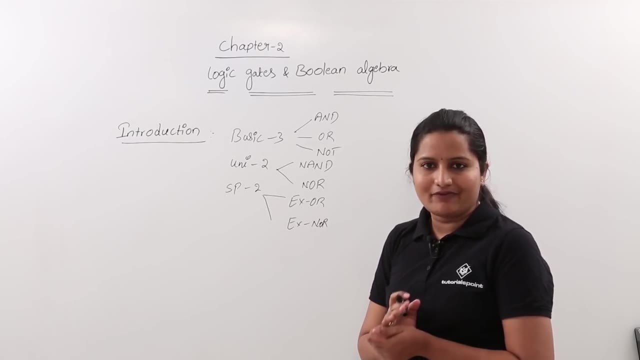 having seven gates AND OR NOT: NAND, NOR, XOR and XNOR. Now we will see the functionality of each and every gate here. Here, if you see this XNOR gate, you can see that XNOR gate is. 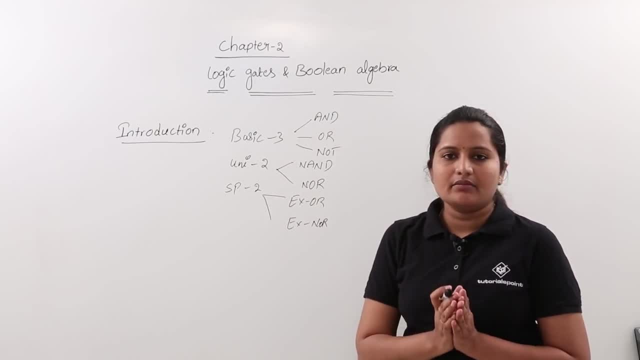 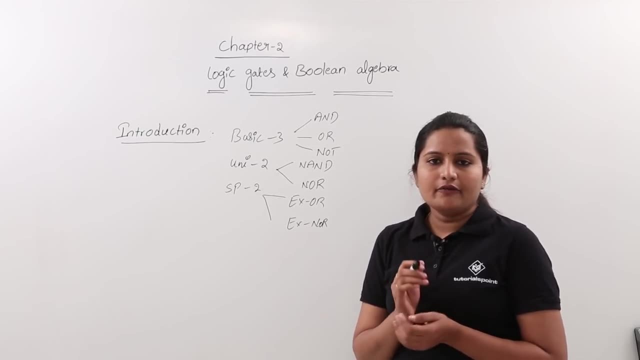 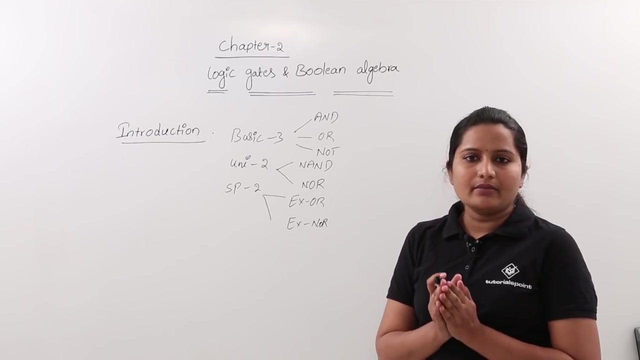 a single gate. So if you are having end gate, means end is nothing but multiplication functionality. You just treat like multiplication functionality. For example, if you are having two input end gate, you may have N input end gate. but for example- I am taking diagram: 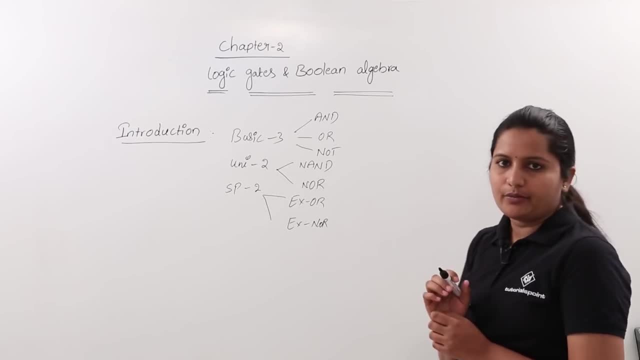 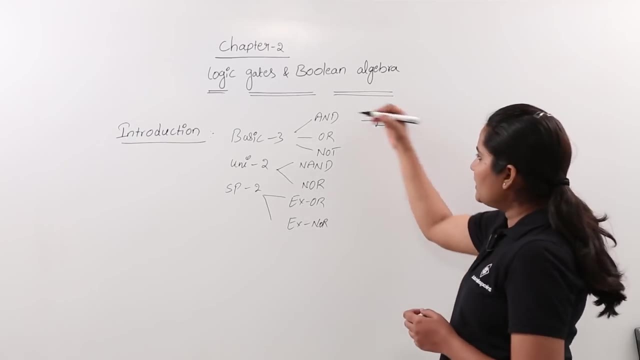 or logic symbol for end gate for two input. So here this is logic symbol for end gate With two pre lines. So this is AND gate with two inputs, some A and B I am taking. inputs are A and B. you can take any name for inputs and here output. I am taking some Y here. So 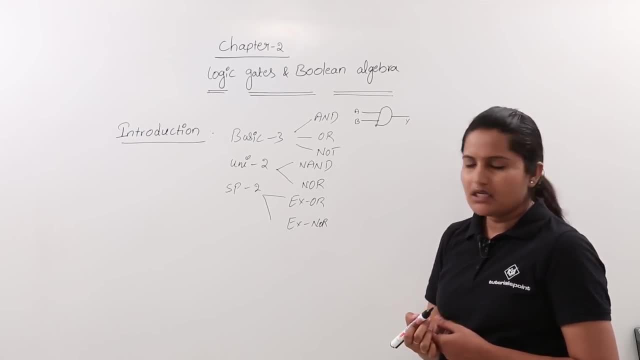 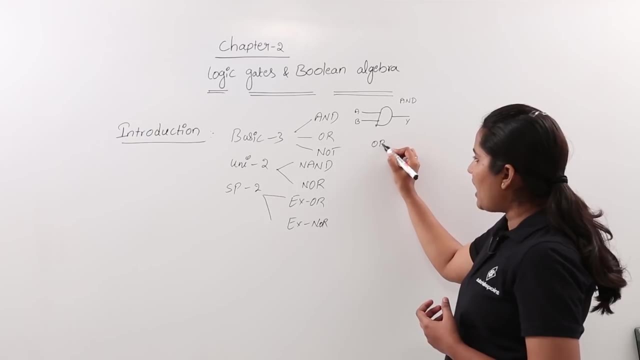 now the logic symbol for this is logic symbol for AND gate. The logic symbol for R gate. I am taking the logic symbol for two input: R gate is N jetzt XNO gate. I am taking N gate. This is using the specific logic symbolethis is specific symbol for A and B. Now, if you 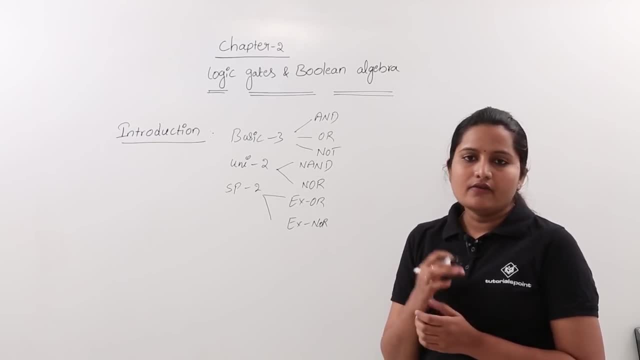 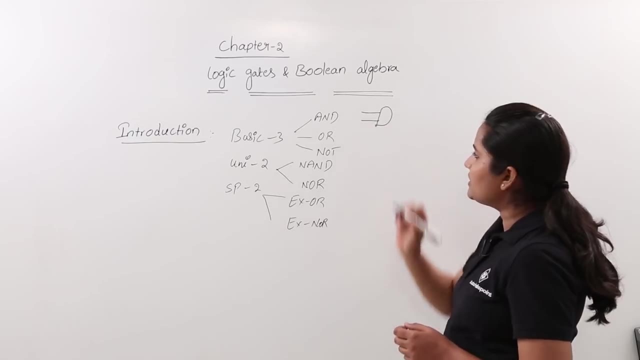 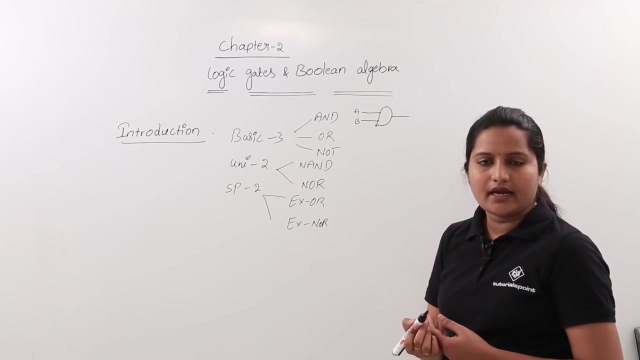 I am taking diagram or logic symbol for NAND gate for two input. So here this is logic symbol for NAND gate. This is I am taking or logic symbol with two prelines. So this is and gate with two inputs, some A and B. I am taking inputs or A and B, you can take any name for inputs. and here 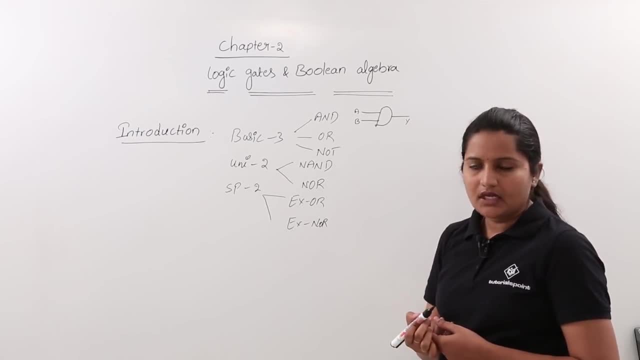 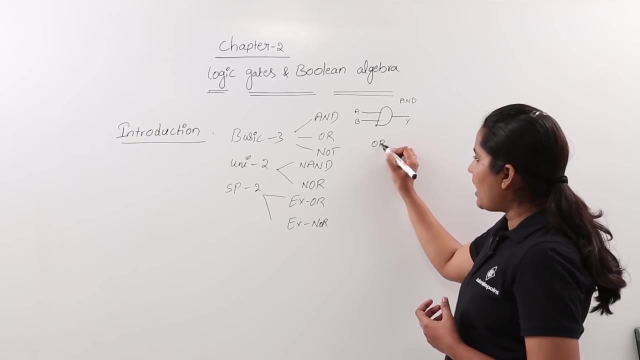 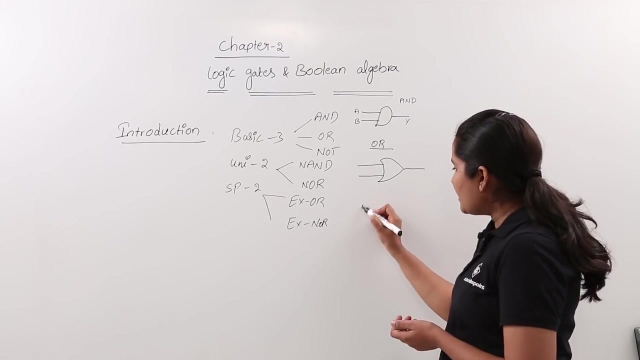 or output. I am taking some Y here. So now the logic symbol for this is logic symbol for AND gate, the logic symbol for OR gate. I am taking The logic symbol for two input gate will be like this: This is symbol for R gate. So in the same way for NOT gate, the logic symbol. 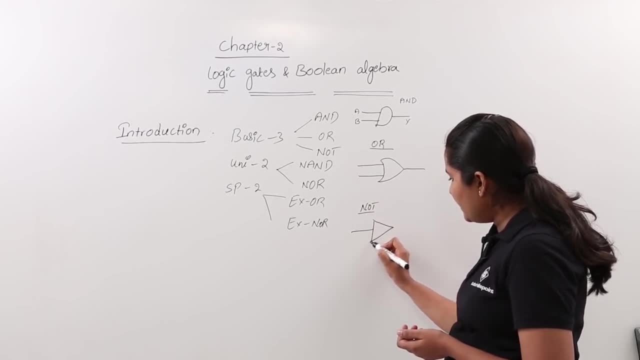 will be so like this. This will be like this. So you are just putting a NOT for buffer. So you know that this is a diode like symbol, but here you are putting NOT. So this is NOT gate, As you are giving some X or A as input. you are getting some X bar at output, For example. 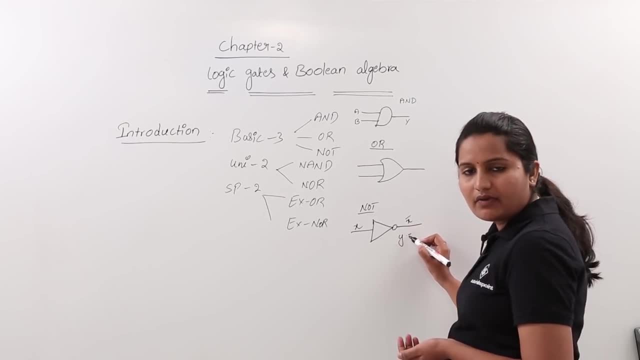 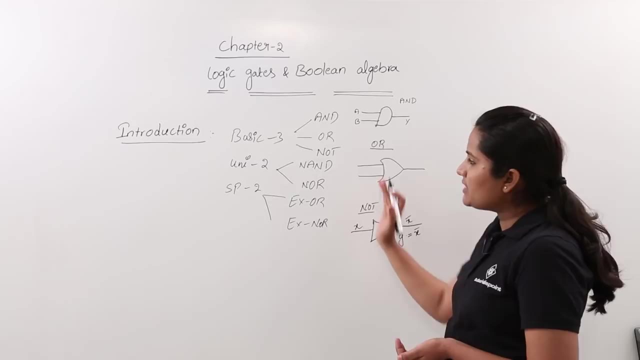 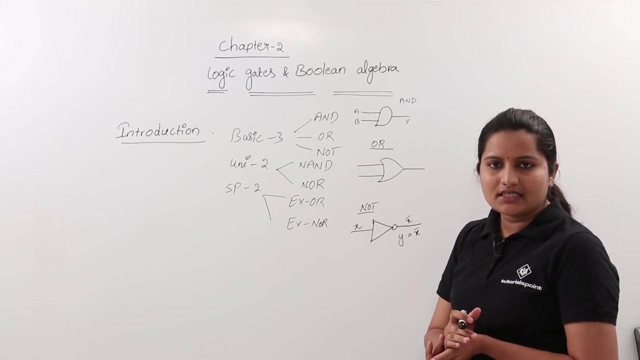 if Y is the output at, NOT gate, so this Y is nothing but complement of input. that means X bar you are going to get. So these are the logic symbols for basic gates. Now we will go for what are the logic symbols for universal gates? that is NAND and NOT. 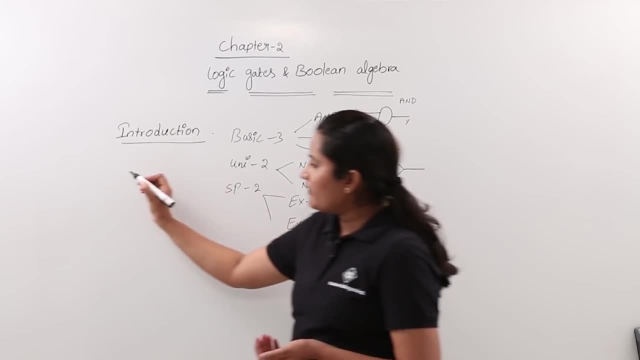 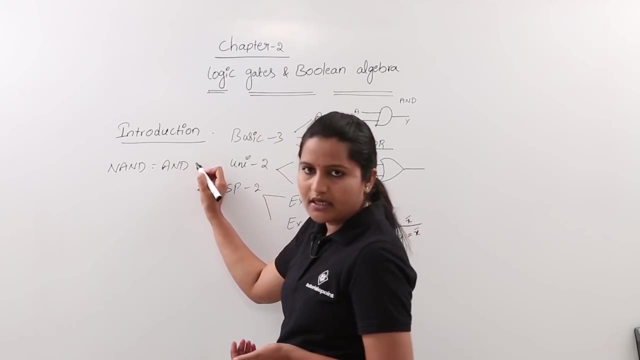 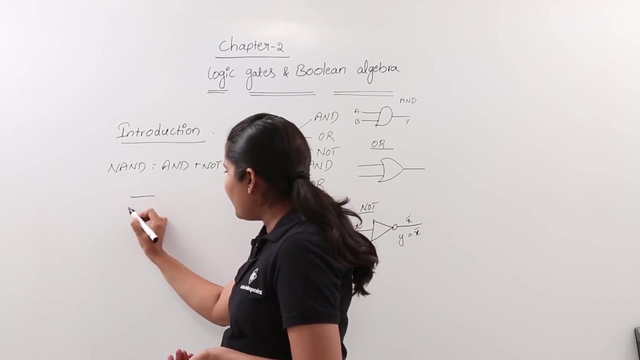 Here NAND is nothing but NAND gate. So NAND gate is nothing but NAND gate. So NAND gate is nothing but. So here we can say: NAND is equal to AND with NOT. AND plus NOT is nothing but NAND. So we know that this symbol for logic, symbol for AND gate, So this is logic symbol for AND gate. 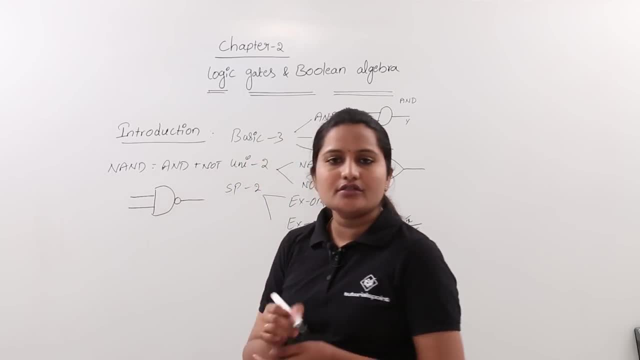 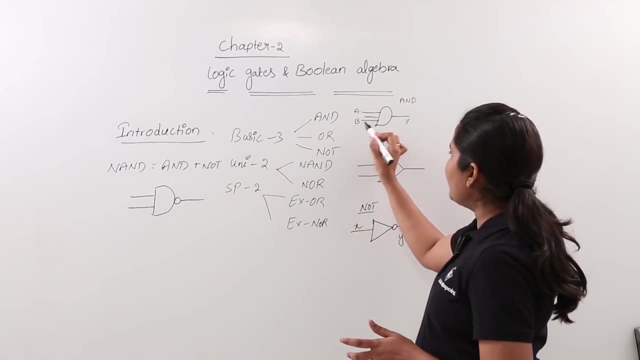 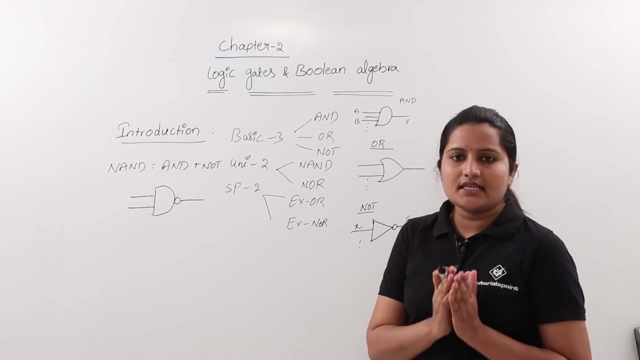 If you take in a NOT here, then you are going to get the symbol for NAND gate. So all I am taking for two input. You may have N input, You may have N input gate, but the symbol is same, The number of lines at. 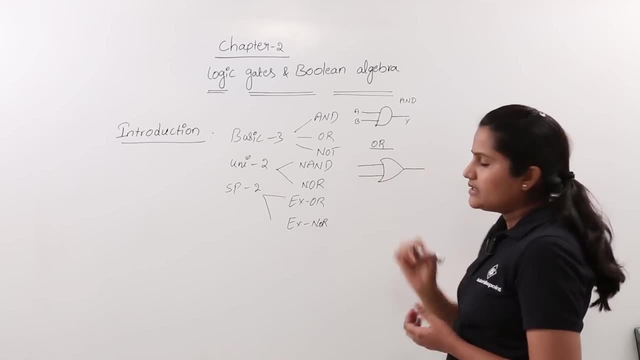 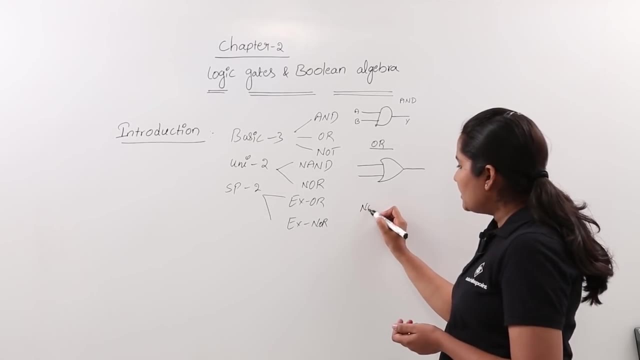 start taking right side fields respectively. P has a particular function, so this is one will be like this: This is symbol for R gate. So in the same way, for NOT gate, the logic symbol will be so like this: This will be like this: So you are just putting a, NOT for buffer, So 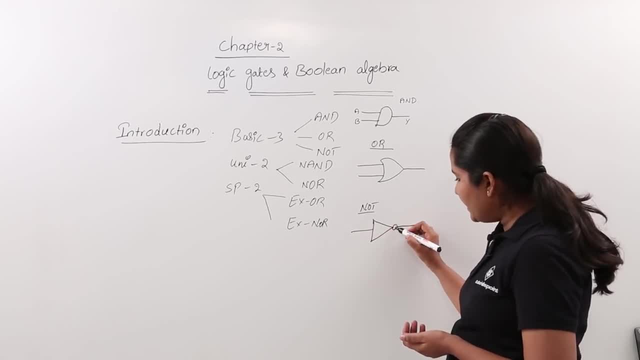 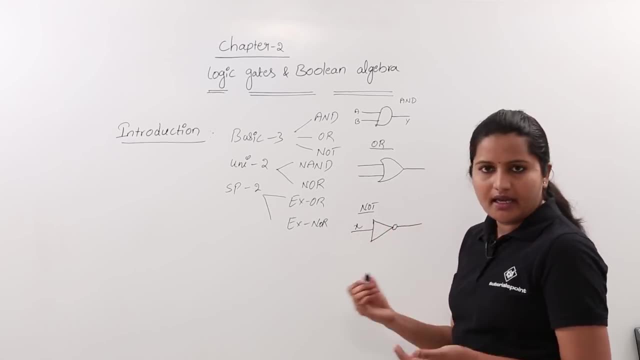 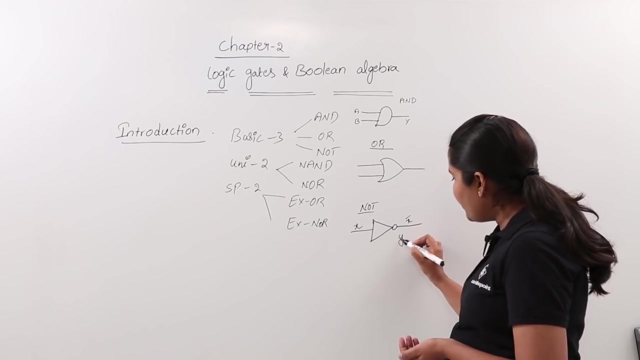 you know that this is a diode like symbol, but here you are putting NOT. So this is NOT gate, As you are giving some X or A as input, you are getting some X bar at output, For example, if Y is the output at, NOT gate. so this Y is nothing but complement of input. that means 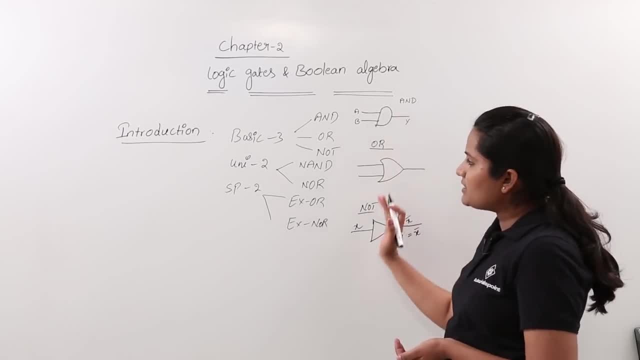 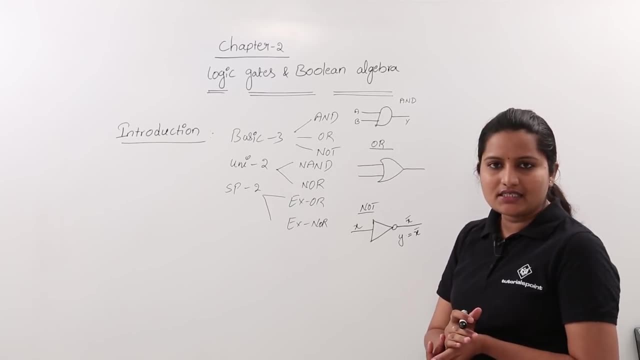 X bar you are going to get. So these are the logic symbols for basic gates. Now we will go for what are the logic symbols for universal gates? that is NAND and NOT Here. NAND is nothing but NAND gate, So NAND gate is nothing but NAND gate. So NAND gate is. 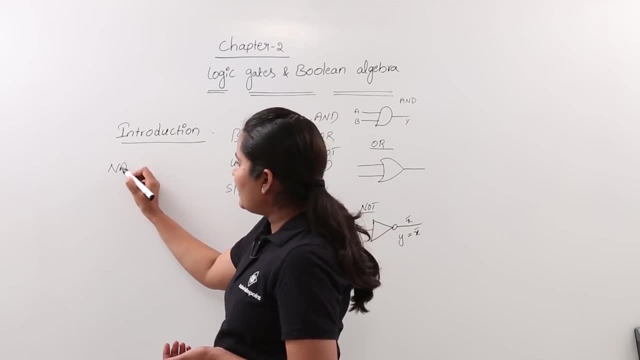 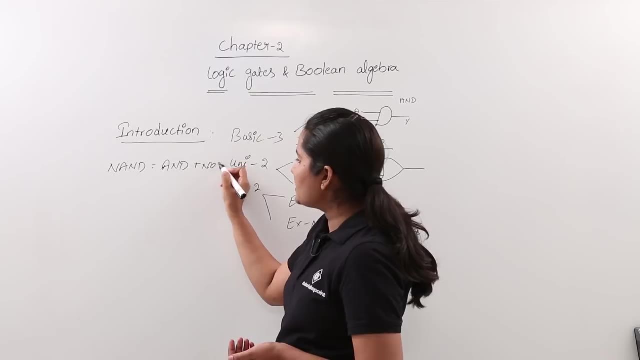 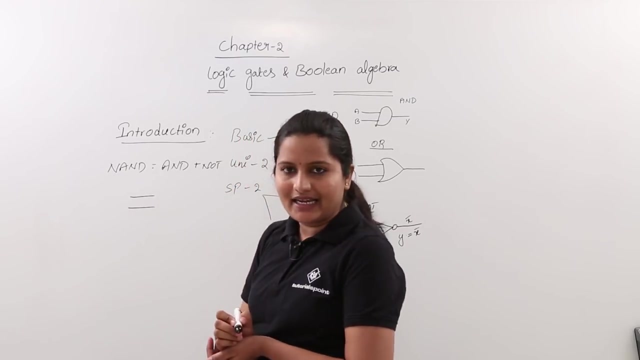 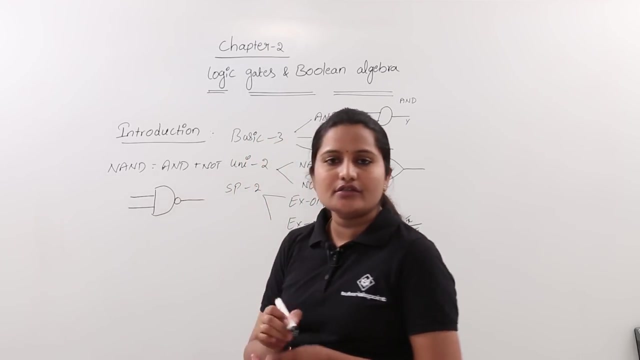 nothing but. So here we can say: NAND is equal to AND with NOT. AND plus NOT is nothing but NAND. So we know that. this symbol for logic, symbol for AND gate. So this is logic symbol for AND gate. If you take in a NOT here, then you are going to get the symbol for NAND gate. So all I am taking 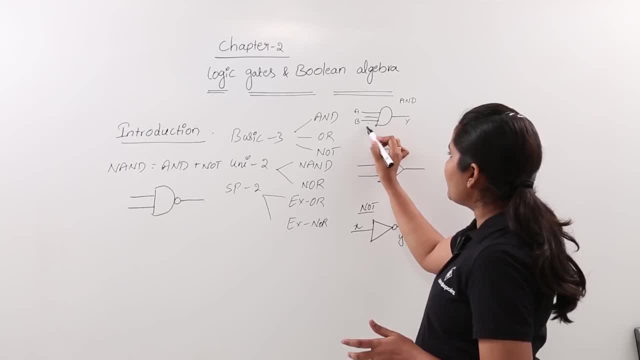 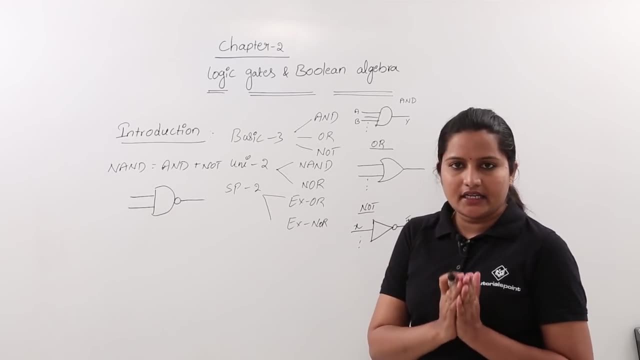 for two input. You may have N input, You may have N input gate, but the symbol is same. The number of lines at input may vary. All gates are having only one output Only. the difference between N input AND gate or N input gate and two input gate is number of input lines. So here this is two input, NAND. 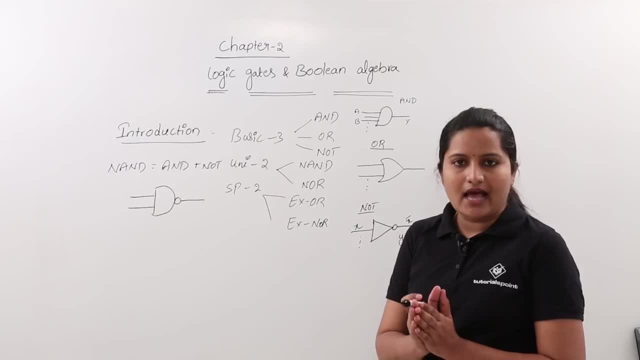 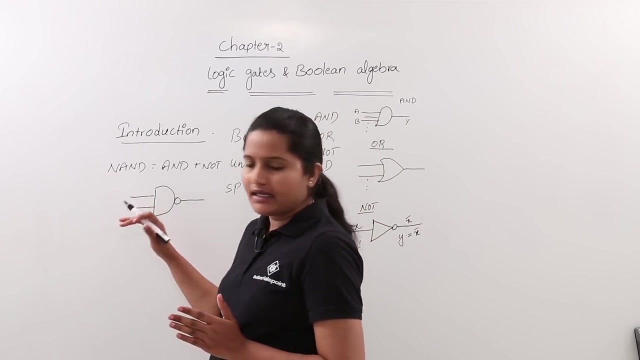 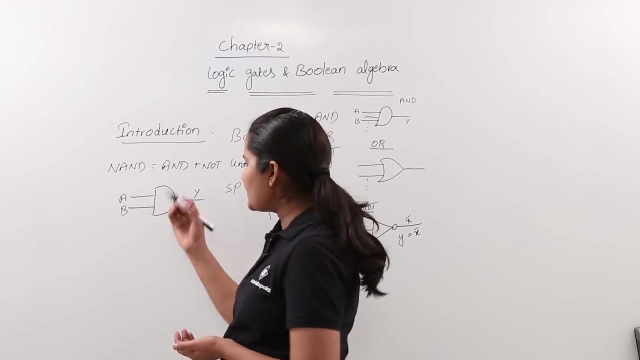 input may vary. All gates are having only one output Only. the difference between N input AND gate or N input gate and two input gate is number of input lines. So here this is two input, NAND gate. Here only two input and 1 output. So similarly so, here NOR gate is equivalent to R plus NOT So R followed by NOT. 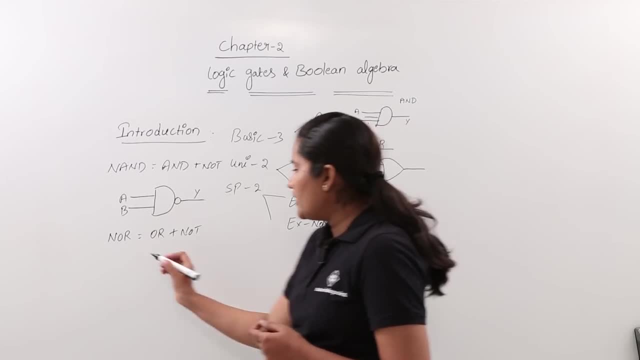 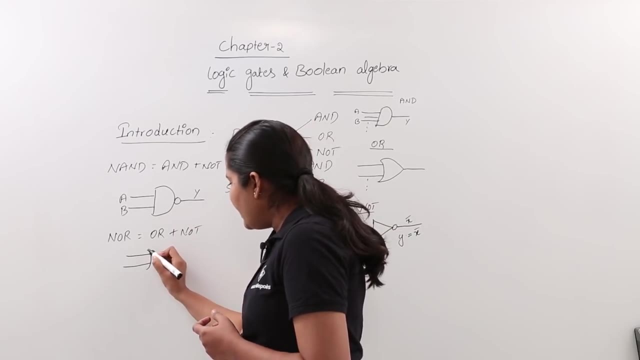 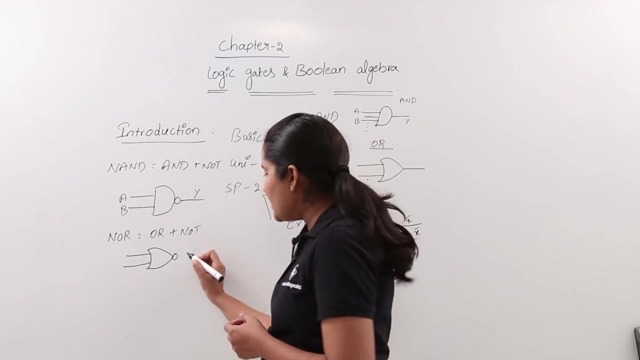 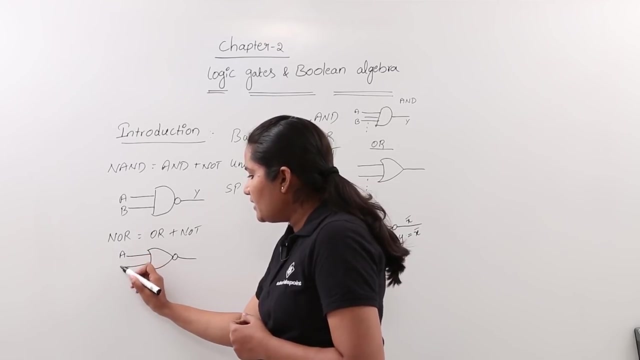 is nothing but NOR gate. So here the logic symbol for NOR gate can be drawn. like you know, R gate and you just need to take a NOT for this R gate. So this is the symbol for NOR gate. So this is the logic symbol for NOR gate, and here the input lines are A and B, here output: I am. 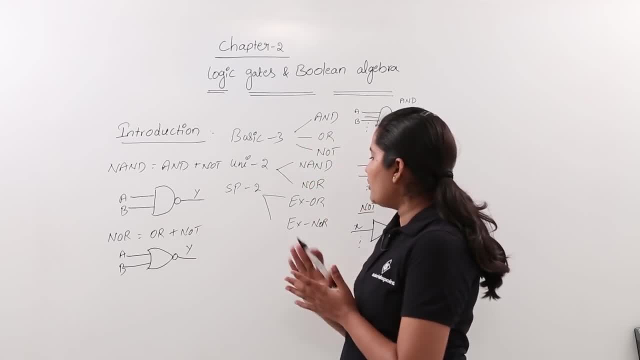 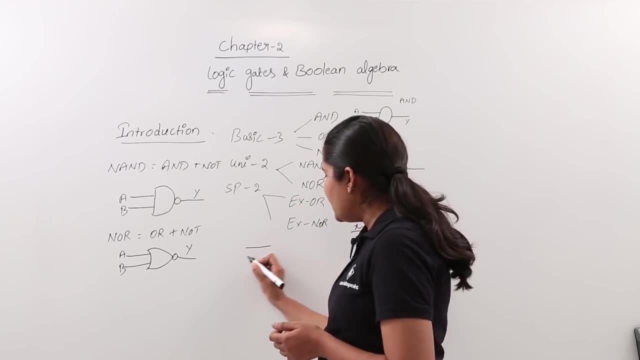 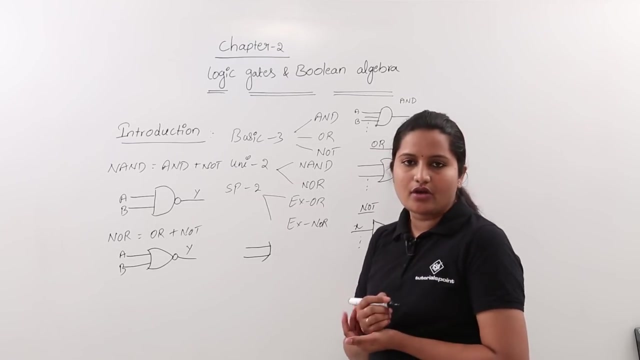 taking like Y. So now we will go for this special gates, that is, XR and XNR. So this XR gate can be XNR, Exclusive R gate. this XR is also called as exclusive R gate. Here this gate can be represented. 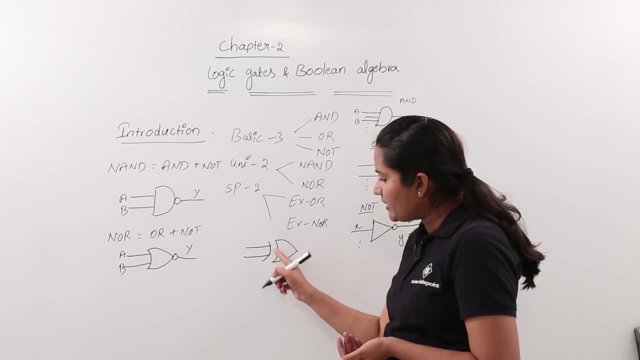 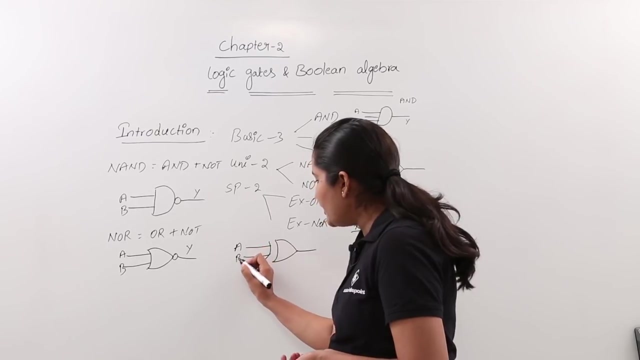 like this in type of R gate only, but we are taking a curve in front of that to get the input lines, So it is having it here also. I taken 2 input XR gate. we may have N input XR gate. Here also I am having 2 inputs and 1 output. As I told you, XNR is somewhat. 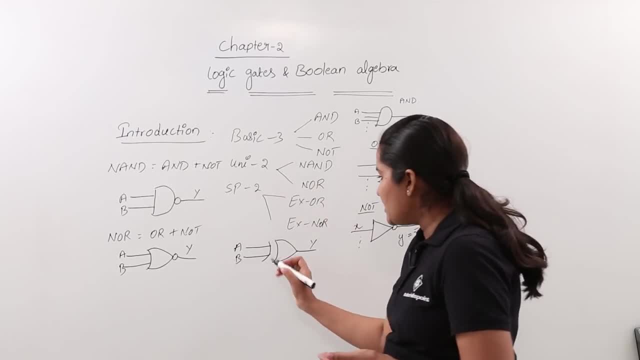 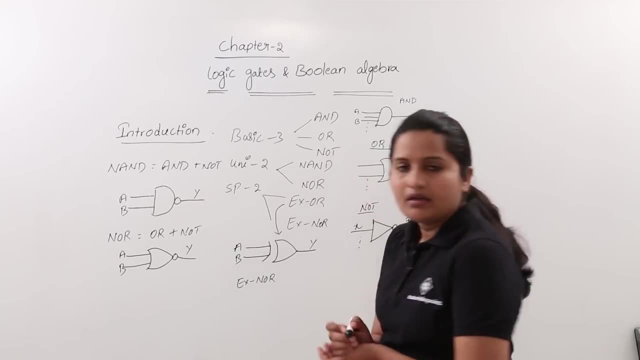 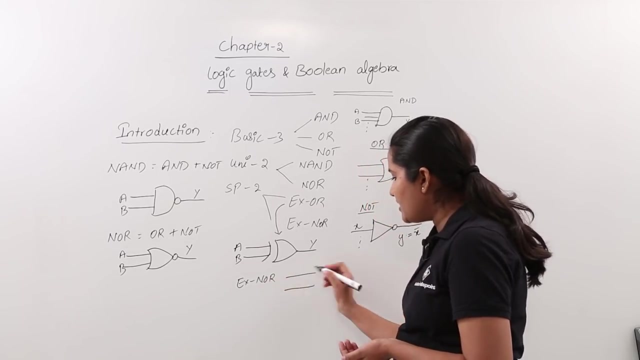 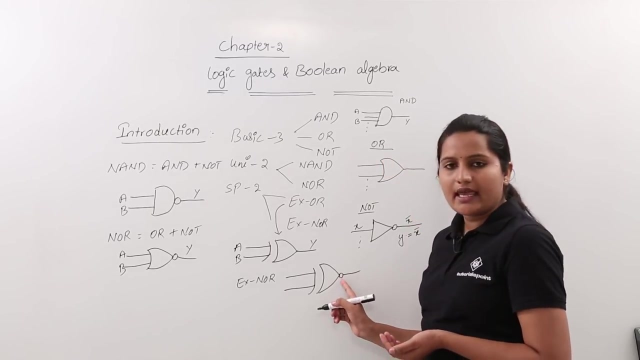 complemented gate for XR, So the symbol for this is symbol for XR. the symbol for XNR can be taken by taking bubble at the end of XR gate. That means so the symbol for XNR gate is so XR gate bubbled, then it is going to produce XNR. This is also having 2 inputs and 1 output. So 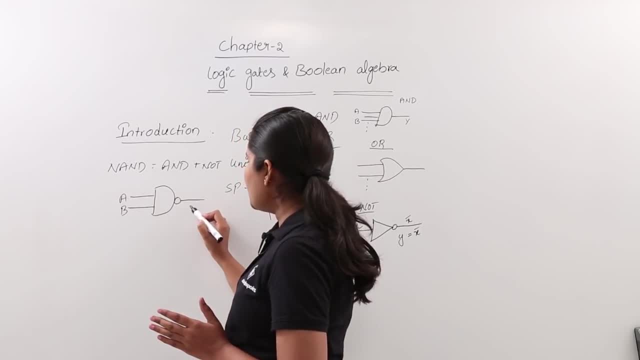 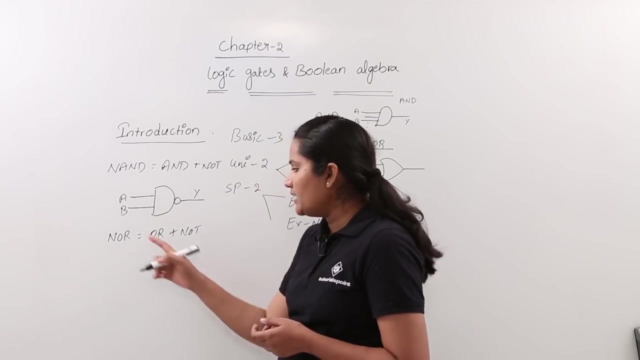 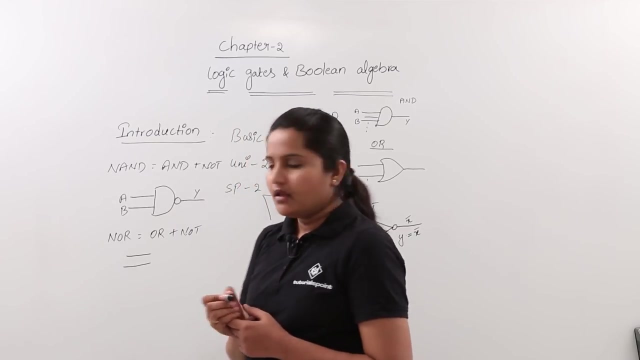 gate Here only two input And one output. So similarly. So here NOR gate is equivalent to R plus NOT. So R followed by NOT is nothing but NOR gate. So here the logic symbol for NOR gate can be drawn, like you know, R gate and. 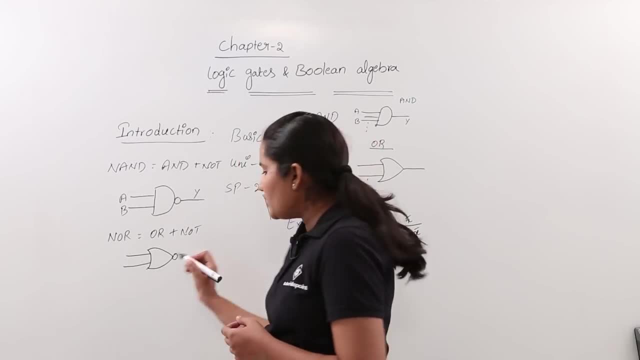 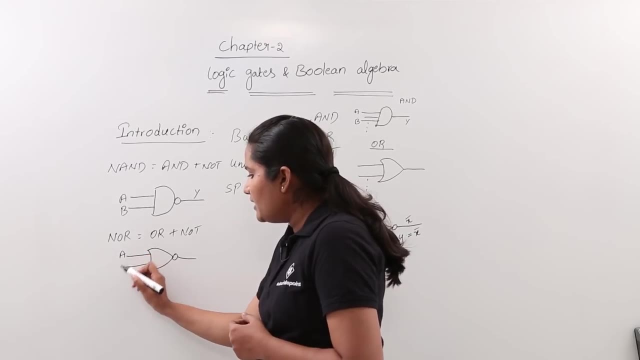 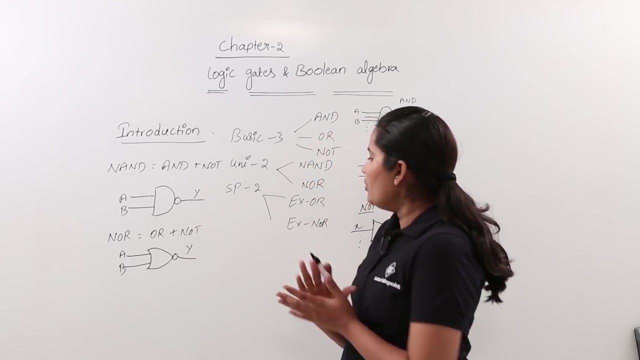 you just need to take a, NOT for this R gate. So this is the symbol for NOR gate. So this is the logic symbol for NOR gate, And here the input lines are A and B, Here output I am taking like Y. So now we will go for this special gates, that is, XR and XNR. 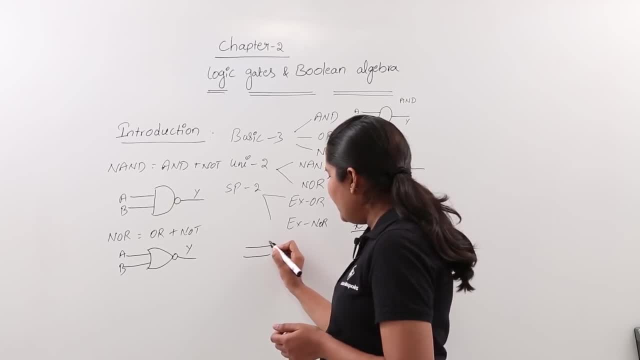 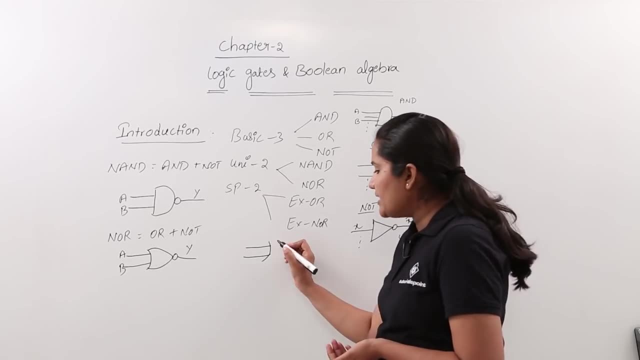 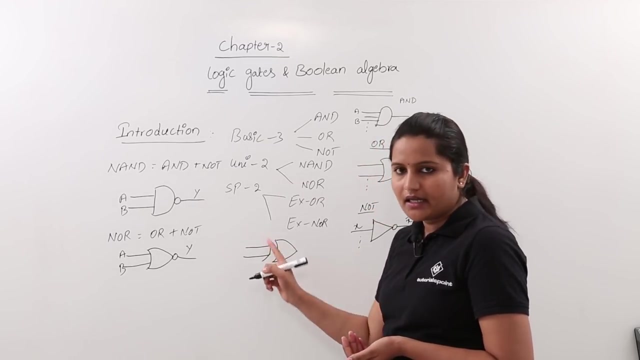 So this XR gate can be exclusive R gate. This XR is also called as exclusive R gate Here. this gate can be represented like this in type of R gate only, but we are taking a curve in front of that to get the input lines, So it is having it here also. I taken 2 input. 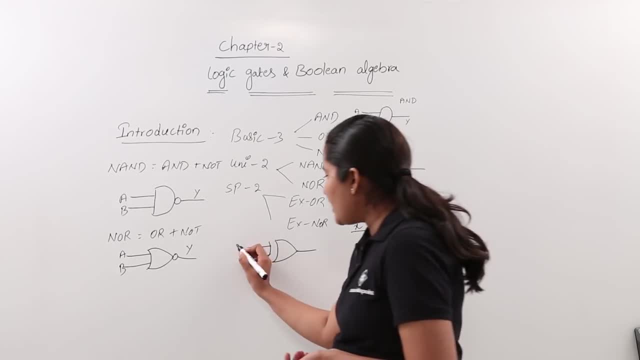 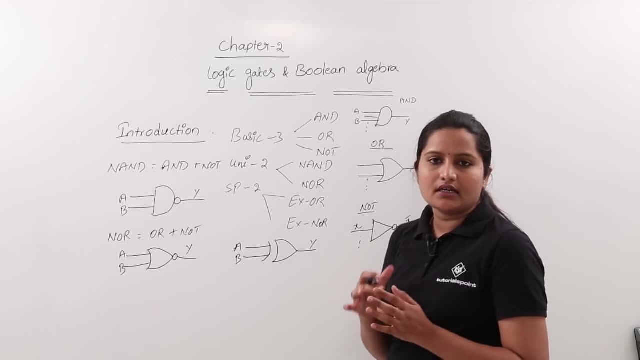 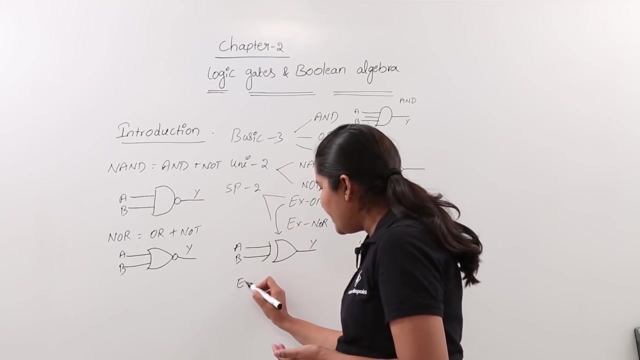 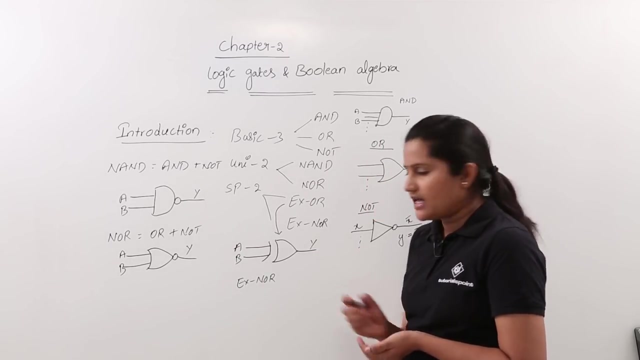 XR gate. we may have N input XR gate. Here also I am having 2 inputs and 1 output. As I told you, XNAR is somewhat complemented gate for XR, So this symbol for this is symbol for XR. the symbol for XNAR can be taken by taking bubble at the end of XR gate. That 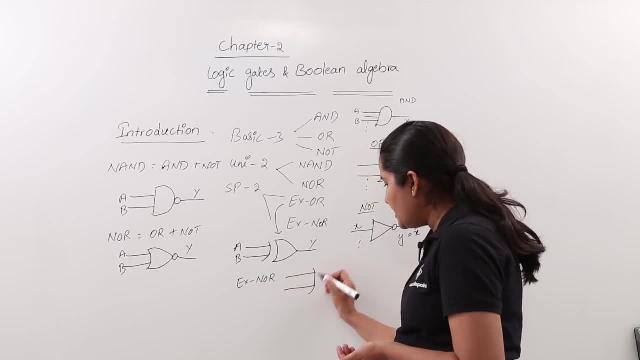 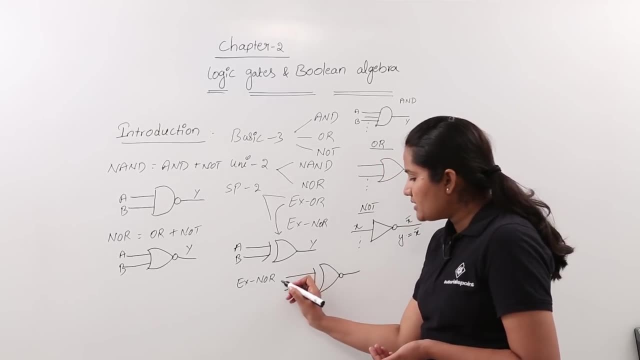 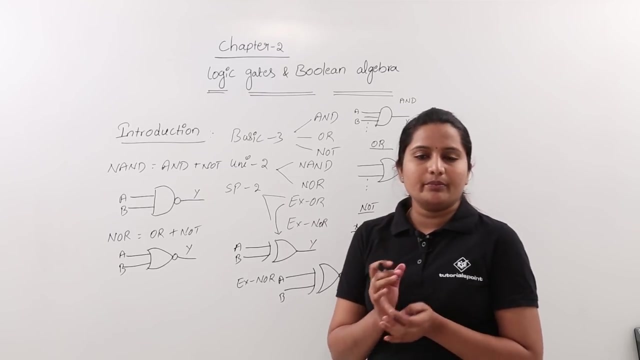 means so the symbol for XNAR gate is so XR gate bubbled, then it is going to produce XNAR. This is also having 2 inputs and 1 output. So here logic gates are generally used to implement any logic function. 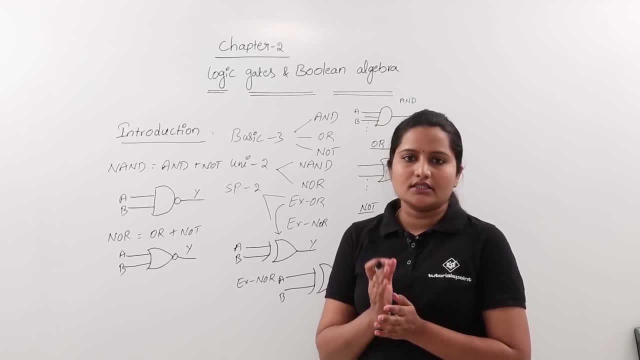 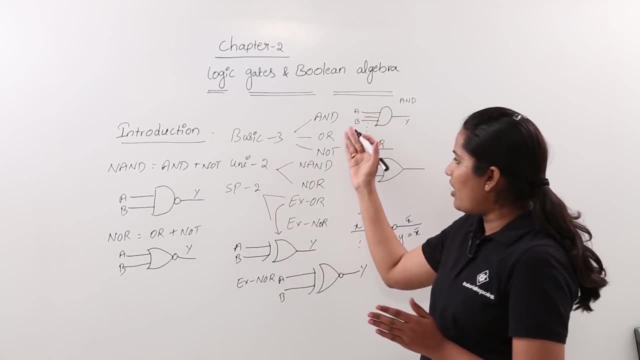 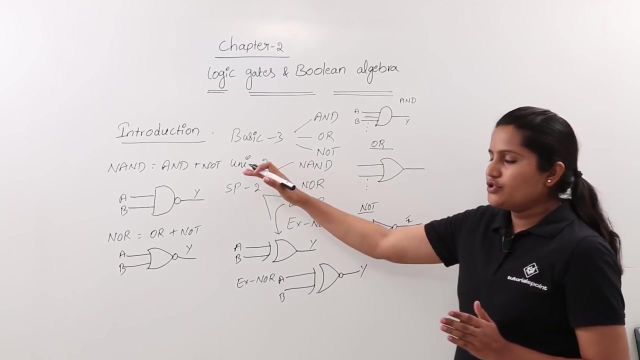 So it performs operations on one or more logic inputs and produces only one output. Here we are having 3 basic gates as AND OR NOT. These are the logic symbols for AND OR NOT. and then we are having 2 universal gates, NAND and NOR, which are nothing but AND plus NOT.